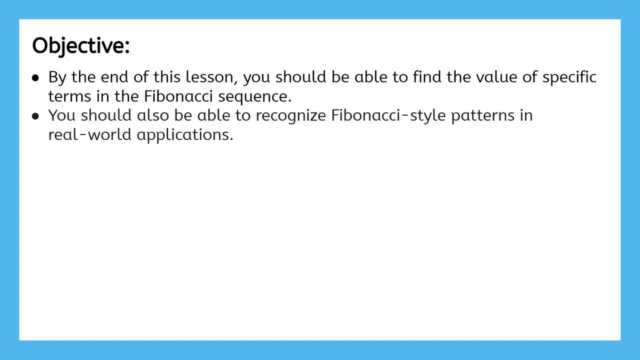 terms in the Fibonacci sequence, You should be able to recognize Fibonacci-style patterns in real-world applications. First we'll discuss the Fibonacci sequence, Next we'll discuss the Fibonacci spiral and the golden ratio And finally we'll discuss more applications. 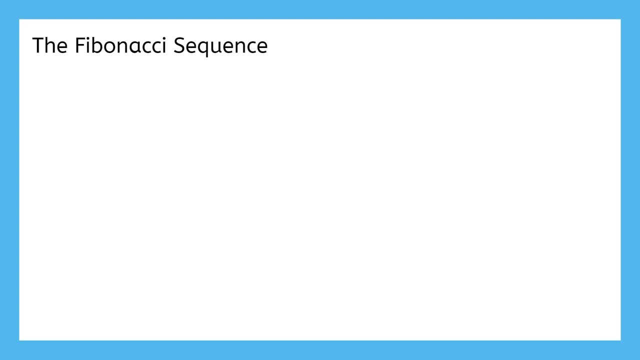 The Fibonacci sequence is an interesting sequence that you may have encountered previously. It's defined by the following formula. Notice that there are two previous terms given. Remember: a sub n minus 1 is the previous term and a sub n minus 2 is the term before that. We've been given the first term, a1, and the second. 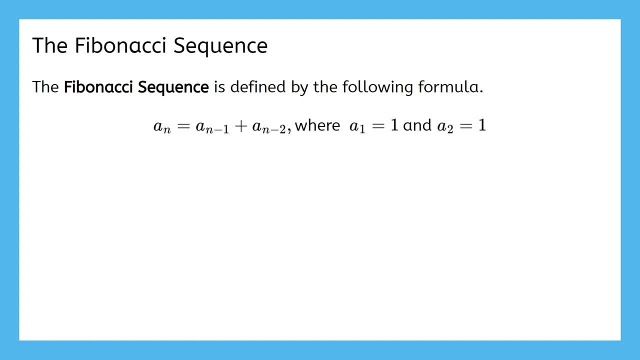 term a2.. And we'll need to find both of those to find a3.. Let's try to find it. the third term According to the formula a3 must be a2 plus a1.. We substitute the appropriate values. Notice. 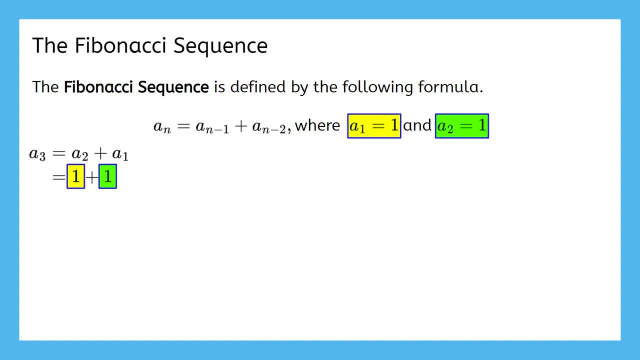 that I switched a1 and a2, as that that's generally a bit easier. with this sequence We find that a3 equals 2.. So here's our sequence so far. Notice that we did 1 plus 1 to get 2.. For the next number: 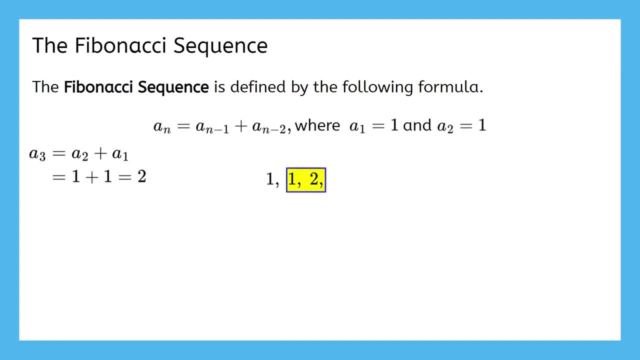 the pattern is the same. We'll take the two numbers, the one we just found and the one before that, to get the answer for a4.. We have 1 plus 2- equals 2.. See equals 3.. Next we'll do 2 plus 3 to get 5, and then this pattern continues. Can you find? 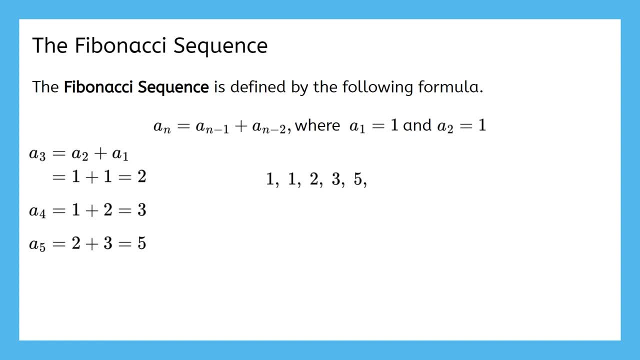 4 more. Pause the video and give it a try. 3 plus 5 is 8,, 5 plus 8 is 13,, and so on. By the way, a formula for the Fibonacci sequence with only numbers and the variable n is really: 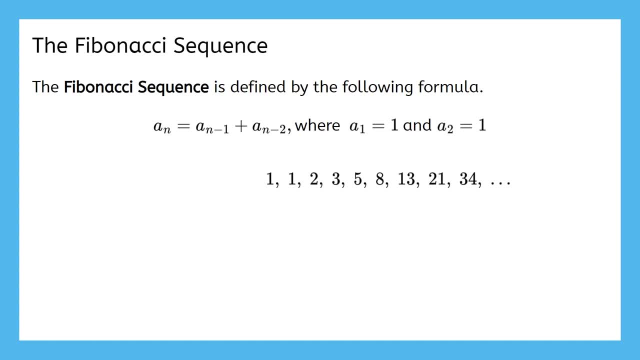 complicated. so if you really want to find a term late in the sequence, you just gotta keep adding. As one final question: what's the 8th term in the Fibonacci sequence? If you've written out the sequence far enough, just count up. 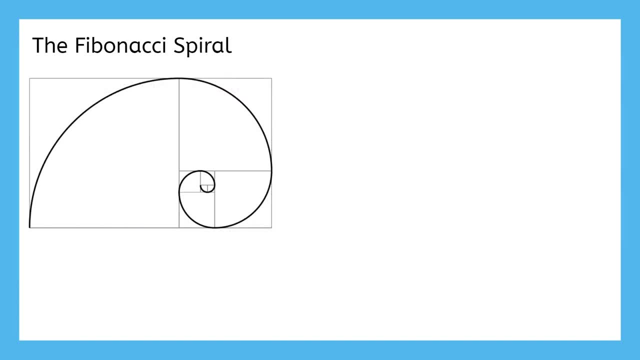 to the 8th one. One reason the Fibonacci sequence is so famous is because it occurs in nature. This is what we call the Fibonacci spiral. Notice how the Fibonacci sequence describes these grey squares' side lengths as they add onto each other. Now check out this Nautilus shell. They match almost perfectly, Isn't that… wild? 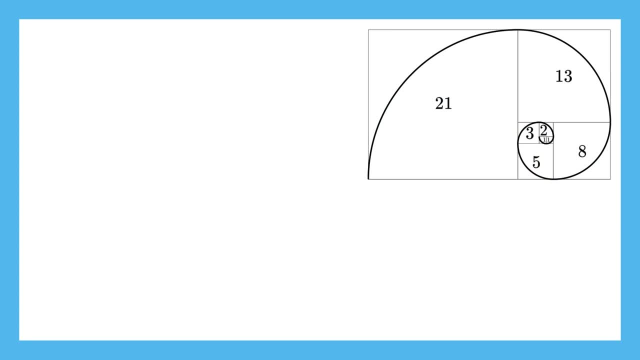 This spiral actually leads to another interesting sequence. Let's look at one piece at a time, specifically at the ratio of its longer side length to its shorter side length. For the first two squares, this ratio is 2 over 1, which is 2.. 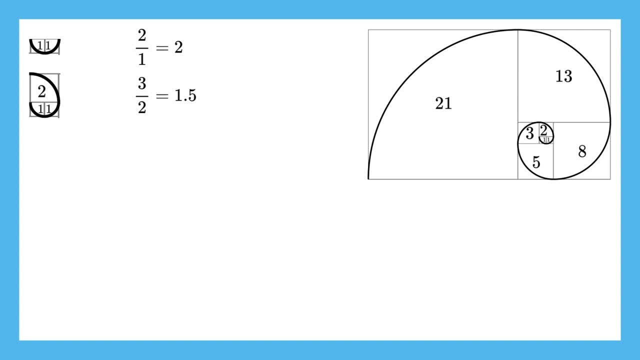 For the first three squares, the long side is now the height, the short side is now the width. Regardless, this ratio is 3 over 2, which is 1.5.. For the next step, we get 5 over 3,. 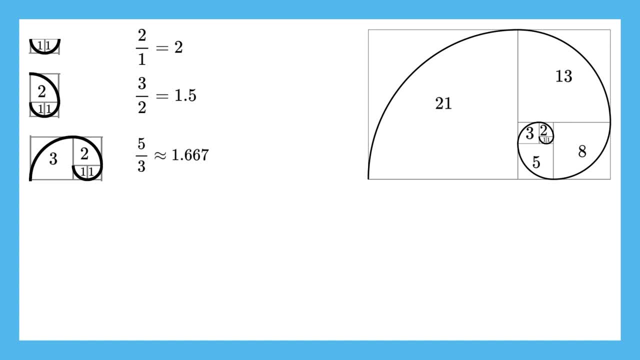 which is about 1.667, repeating. Let's look at one more step. This one is 8 over 5,, which is 1.6.. Now take a look at these fractions. Pause the video and see if you can determine the. 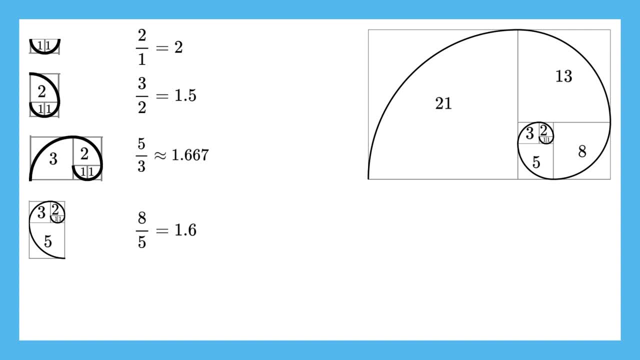 next three fractions. You might even look at the big spiral to make it easier on yourself. Here's our sequence. Notice we're working with the same number of squares, but we're really just dividing consecutive values from the Fibonacci sequence. In addition, you 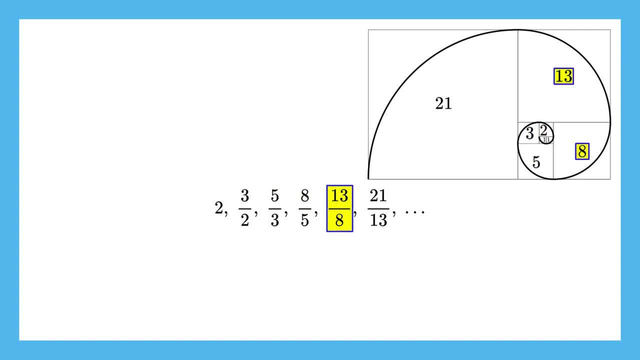 can just grab them right out of the spiral. Now let's write the approximate values for these fractions and see if we notice a pattern. Hmm, They seem to be going up and down, but maybe we should write out a few more terms. It starts repeating. Well, actually it's not, It's just a little bit more than that. 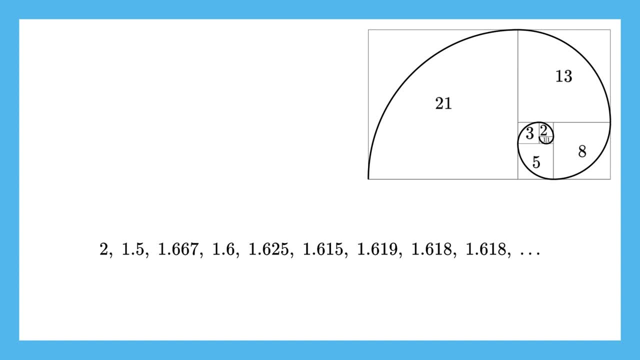 It's a little bit more than that. It's a little bit more than that. It's a little bit more than that. Actually, it doesn't if you don't round, But there must be something special about 1.618.. Let's investigate. 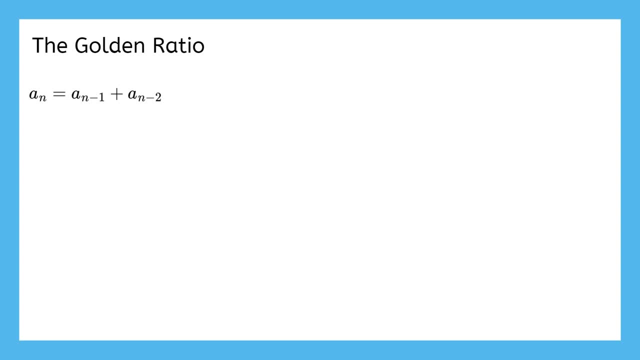 Let's look back at the Fibonacci formula for a moment. We're going to perform some steps that may look odd, but watch until the end, when we'll discover something amazing. We'll replace the furthest-back term a-sub-n-minus-2, with a 1.. The next one, a-sub-n-minus-1, with 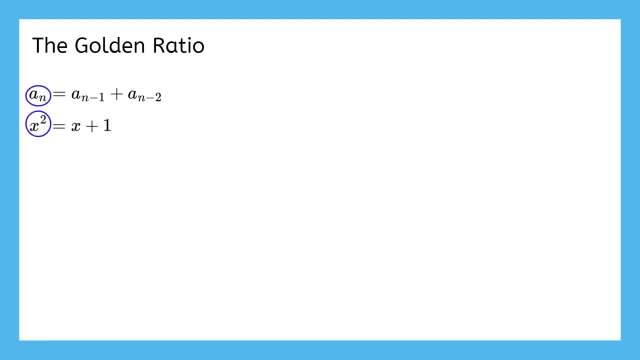 with an x and the current one a sub n, with x squared. To solve this equation, we will set it equal to zero and then use the quadratic formula Simplifying that we get one plus or minus the square root of five all over two. 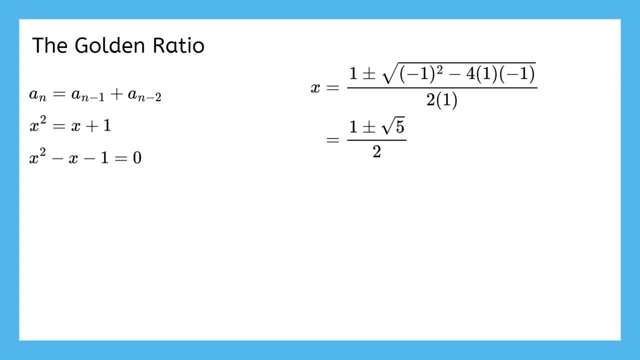 Why on earth did we do this? Well, take a look at the approximation of the solution that uses the plus. Oh, wow, that's the same number that we found on the previous slide. This number is called the golden ratio, named by the Greek letter phi. 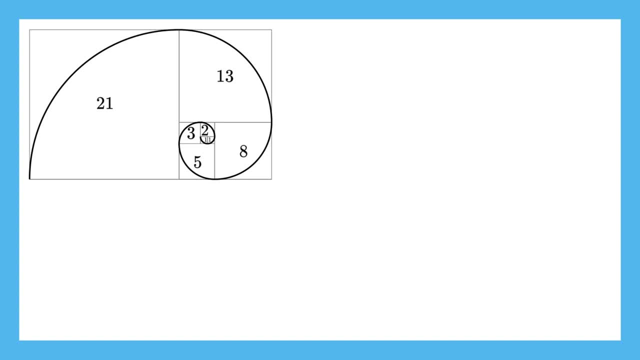 Let's take a look at the spiral again, but now we're going to look specifically at the last rectangle. Do you like this rectangle? I know, I know that's a weird question, but seriously, do you like it? Here's some other rectangles for comparison. 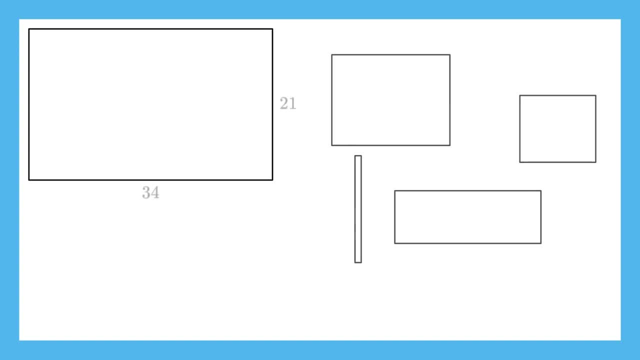 Remember, this rectangle had dimensions 34 by 21, and this ratio was about 1.619.. Almost fine. This is often called the golden rectangle. It's considered to be the most aesthetically pleasing rectangle. It's considered to be the most aesthetically pleasing rectangle. 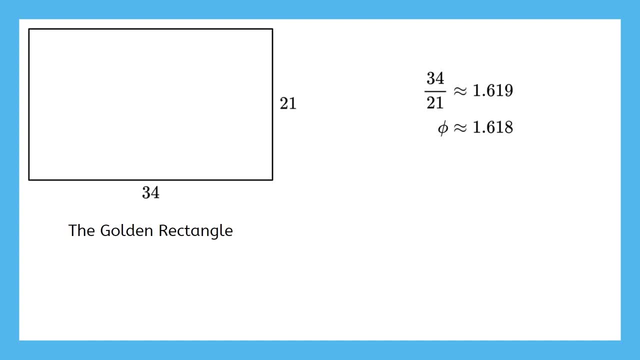 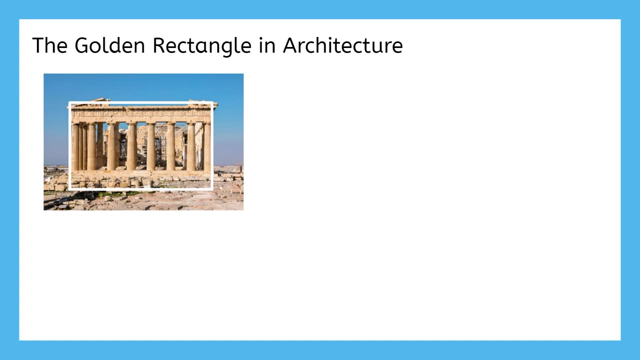 It's considered to be the most aesthetically pleasing rectangle, And it appears in many forms of architecture. And it appears in many forms of architecture. The golden ratio has been known since Ancient Greece and it showed up in their architectural design, such as the Parthenon constructed between 447 and 432.. 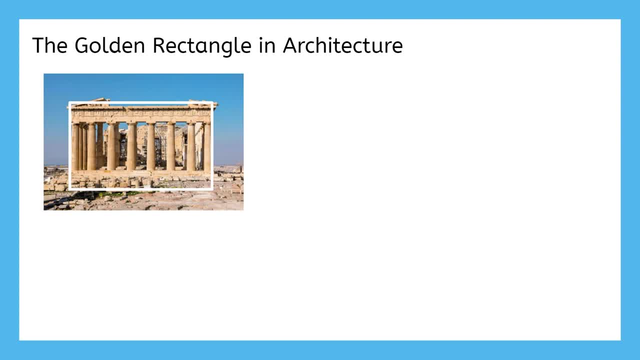 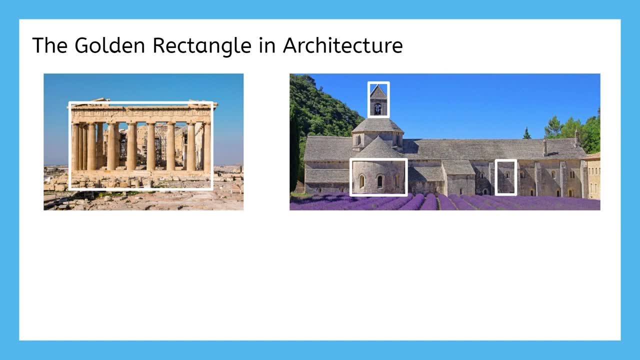 The Golden Ratio was also used in later architecture, such as Romanesque cisternian architecture. This is the Sennonk America found in 1148.. This is the Sennonk America found in 1148.. is used in some modern architecture as well.